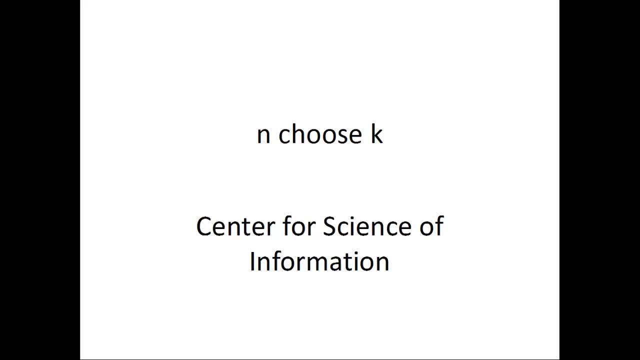 Hello, welcome to the fifth video in the ComTorix module for the Center for Science of Information. Today we'll be talking about the notation we introduced in the previous lecture, the binomial coefficient n, choose k, and some identities associated with it. 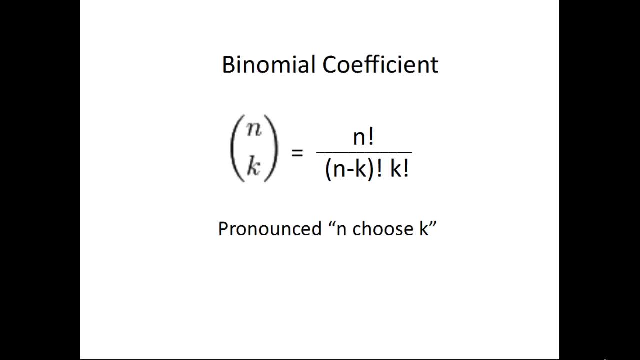 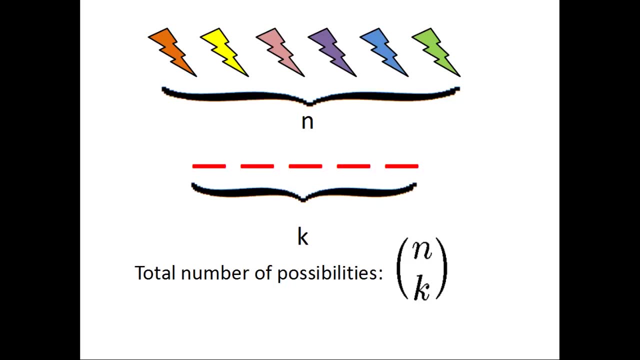 As a reminder, the binomial coefficient pronounced n choose, k equals n factorial divided by n minus k factorial, k factorial, and it represents the total number of possibilities to choose k objects from n total objects. if the order of the objects that we choose does not matter, 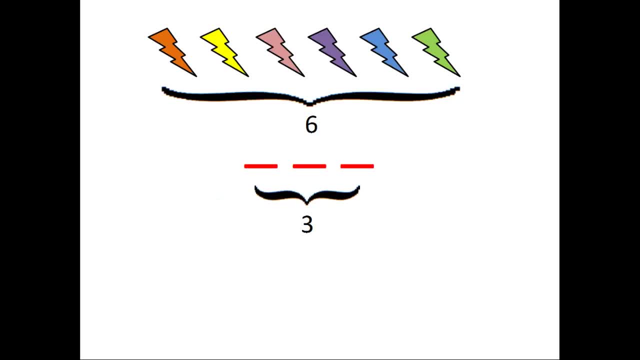 As a warm-up, let's calculate the number of ways to choose three objects from six total objects According to our formula. that is six choose three, which equals six factorial divided by three factorial- three factorial, which equals six times five times four times. 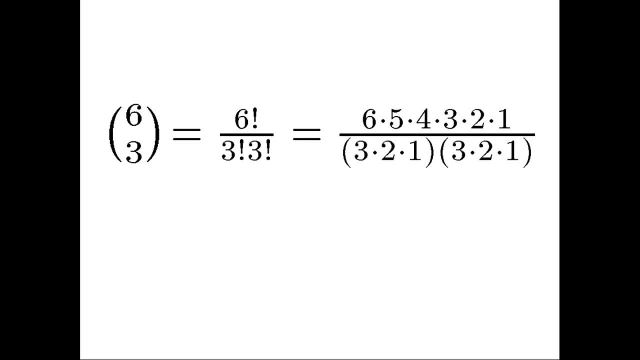 three times two times one, divided by three factorial, three factorial: If we cross out the three times two times one on both the numerator and the denominator, we have six times five times four on the top and three times two times one on the bottom. 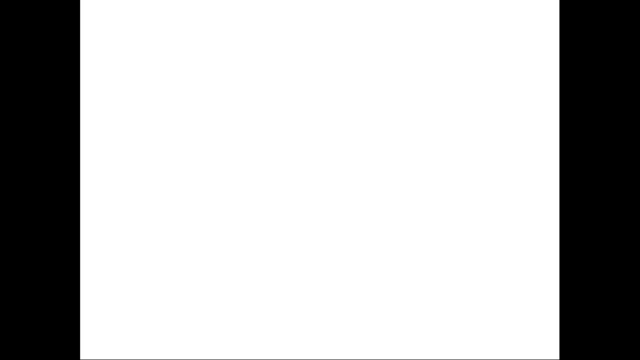 which equals twenty. Now let's look at some identities involving n choose k. First let's take a look at n choose k when n equals six and k equals four. This represents the number of ways to select four objects from a list of objects. 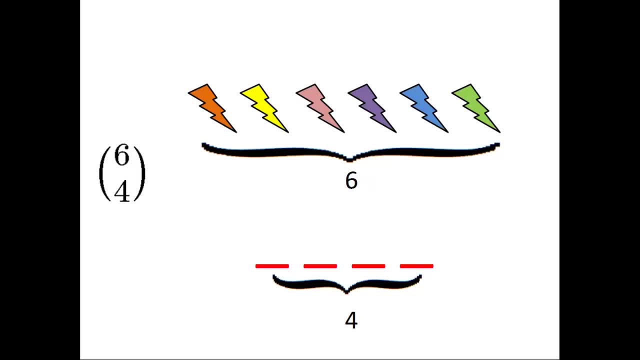 For example, let's suppose we choose these four objects, which is equivalent to choosing two objects to eliminate from the original list. If we eliminate two objects, we'll be left with four objects. so that's another way of choosing the four objects. Hence six. 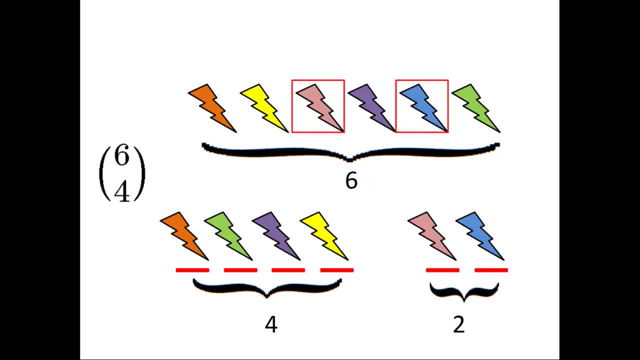 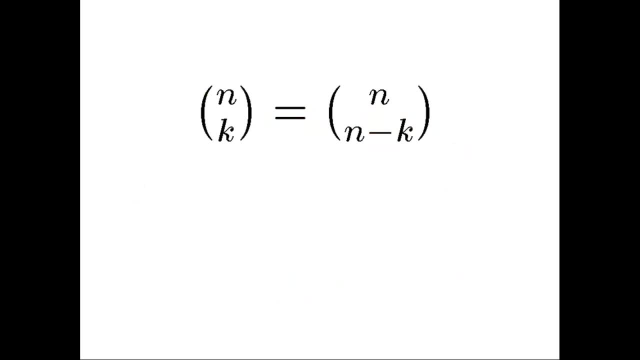 choose four equals six, choose two and, in general, n choose k equals six, choose two. Now let's consider six, choose zero. This equals the number of ways to choose zero objects from six objects. Clearly, there's only one way of doing that, which is choosing none.